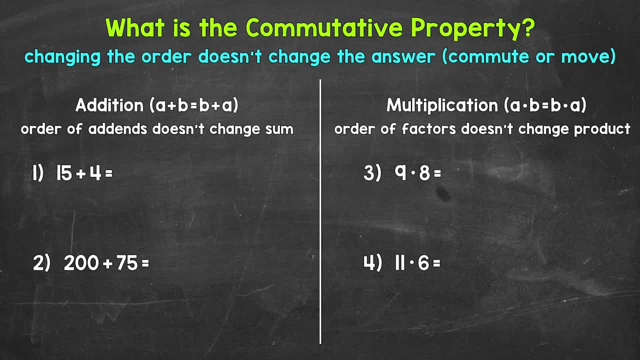 to simplifying algebraic expressions, to whatever else the case may be, The commutative property is important to be familiar with. Now, simply put, the commutative property states. changing the order doesn't change the answer, And we can think of commute or move when it comes to the commutative property. 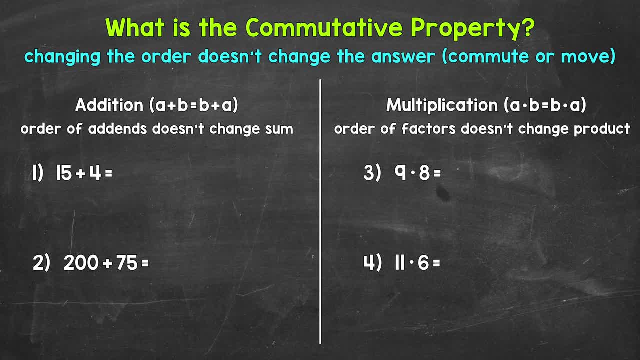 Now, both addition and multiplication are commutative, but subtraction and division are not. We will take a look at all of this as we go through our examples. Let's jump into our examples, starting with numbers 1 and 2, where we will take a look at the commutative property. 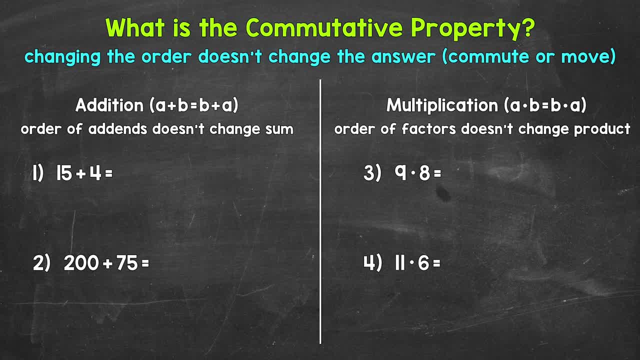 We will look at the commutative property of addition, which states: a plus b equals b plus a. That just means the order of the addends doesn't change the sum. Addends are the numbers that are being added together, And then the sum is the answer to an addition problem. 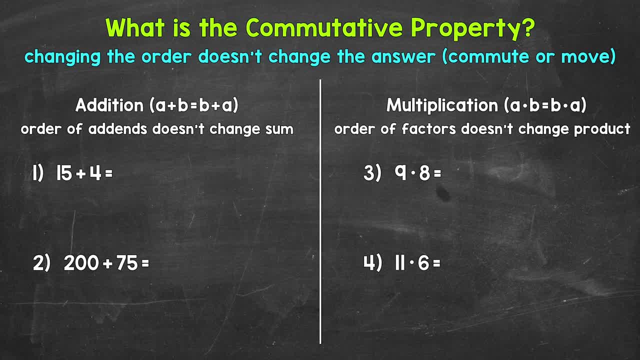 Now don't let the letters confuse you. Those are just there in place of numbers to show that this will work for any numbers. a plus b equals b plus a. b will equal the same exact thing as b plus a. Let's take a look at number 1 and see exactly what this means. 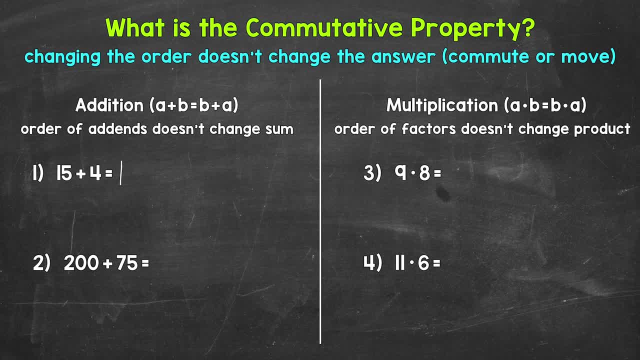 We have 15 plus 4.. That equals 19.. 15 and 4 are the addends, the numbers being added together. 19 is the sum, the answer. The commutative property states that we can change the order. 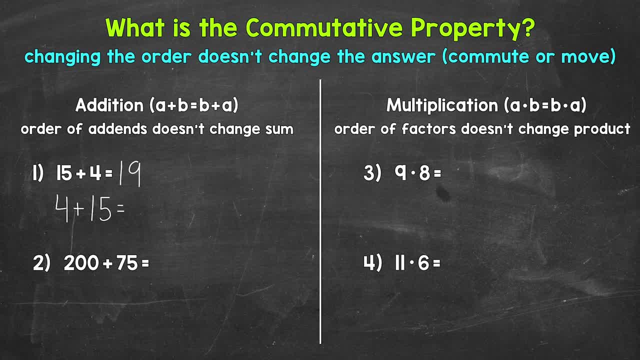 and that will not change the answer. So 4 plus 15 equals 19 as well, And that's the commutative property. 15 plus 4 equals 19.. 4 plus 15 equals 19.. Let's move on to number 2 and take a look at another example of addition. 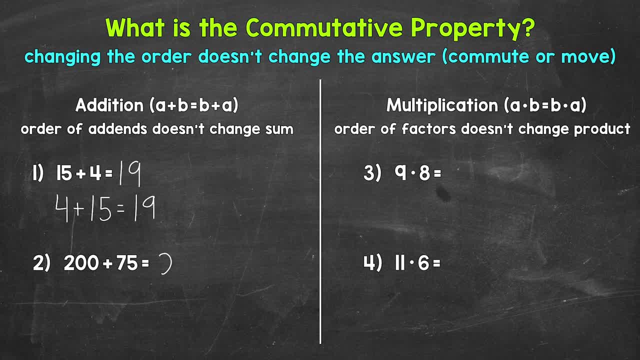 So we have 200 plus 75.. That equals 275.. Change the order: 75 plus 200. And that does not change the answer. So 75 plus 200 equals 275 as well. So to recap: addition is commutative. 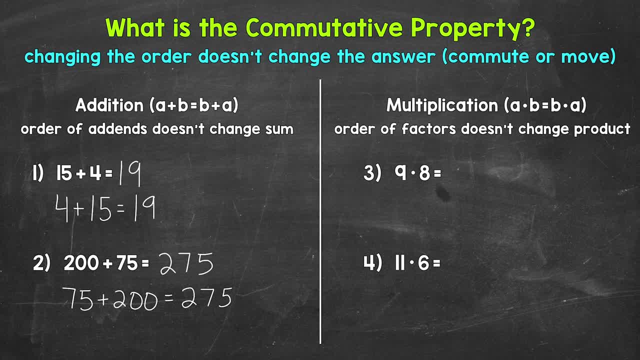 We can change the order of the addends, and that doesn't change the sum. We get the same answer either way. Now let's try this with the inverse of addition, So the opposite of addition, which is subtraction, and see if subtraction is commutative. 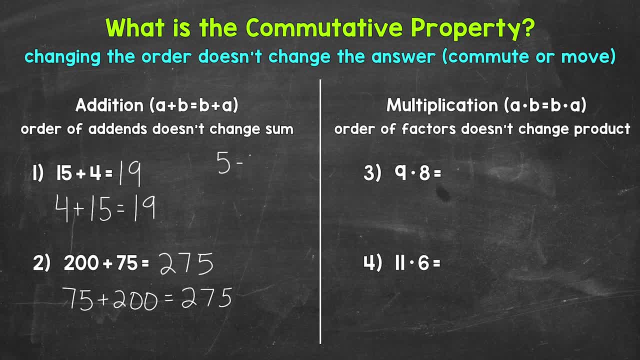 Okay, I'm going to come to the side here. Let's do 5 minus 3, which we know is 2.. Let's change the order: 3 minus 5.. Well, that equals negative 2. So subtraction is not commutative. 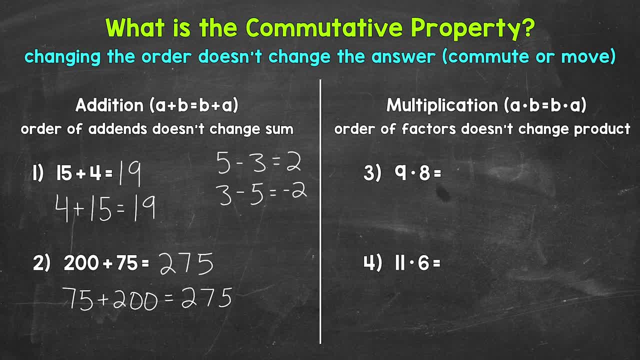 We can't change the order and get the same answer. So again, subtraction, not commutative. Let's move on to numbers 3 and 4, where we are going to take a look at the commutative property of multiplication. 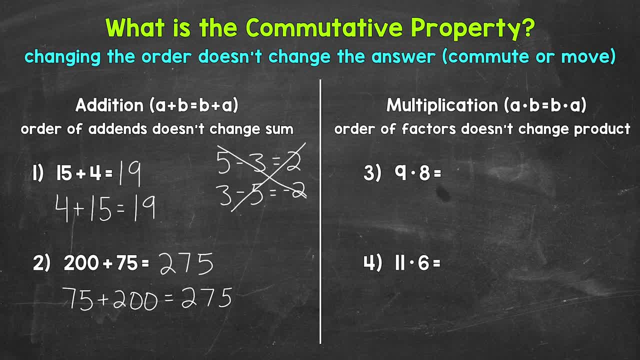 So a times b equals b times a. That just means that the order of the factors doesn't change the product Factors are the numbers being multiplied and then the product is the answer to a multiplication problem. So a times b is going to equal the same exact thing as b times a. 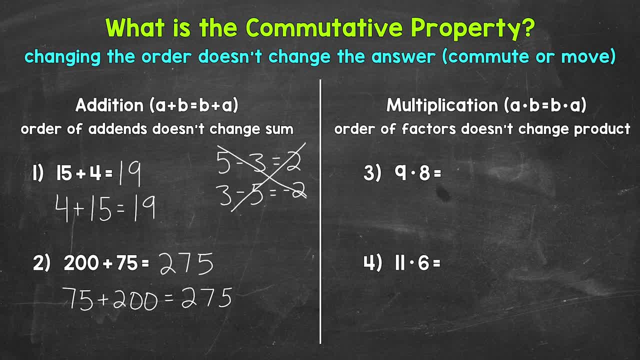 Let's take a look at number 3 and see exactly what this means: 9 times 8.. That equals 72.. Change the order: 8 times 9.. That equals 72 as well. 9 times 8 equals 72, and 8 times 9 equals 72.. 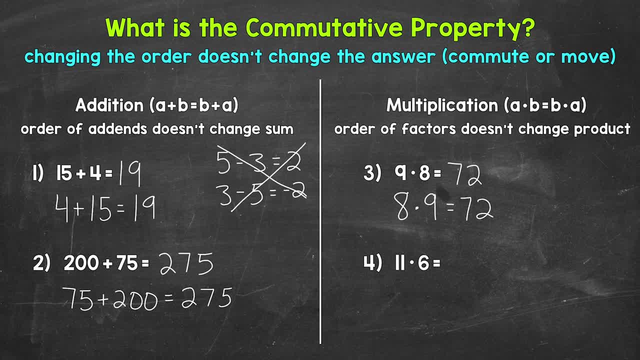 Changing the order didn't change the answer. Order didn't matter. Let's move on to number 4, where we have 11 times 6.. That equals 66.. 66.. Change the order: 6 times 11.. That equals 66 as well. 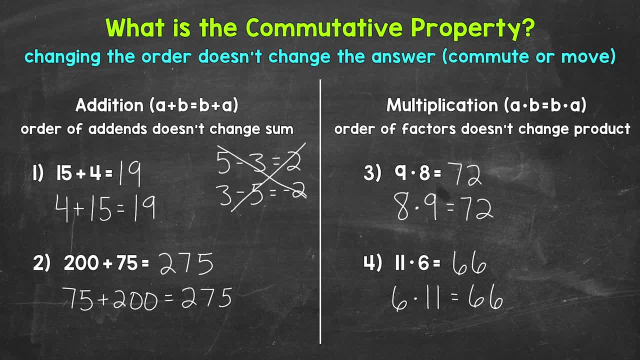 So that's what the commutative property looks like. when it comes to multiplication, We can change the order of the factors, and that doesn't change the product. Now let's take a look at the inverse of multiplication, So the opposite of multiplication, which is division.